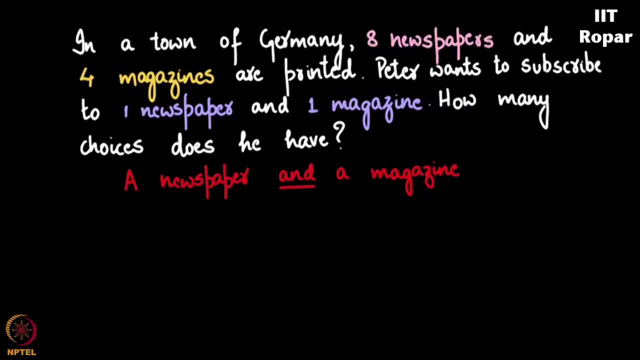 I am stressing upon the word and here because he wants a newspaper and a magazine. So he has 8 newspapers and a magazine. So he has 8 newspapers and a magazine And 4 magazines to choose from. And therefore it is 8 multiplied with 4, which is 32 choices. 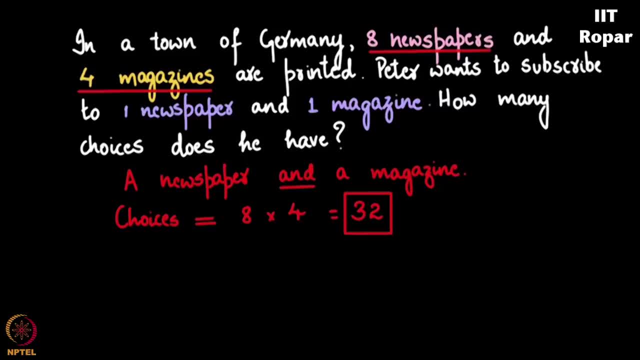 And out of these 32 choices he is going to pick a newspaper and a magazine. Let me just change the question here slightly. Suppose Peter wants a newspaper or a magazine- You see the word- and became or. Here he would have 8 plus 4 choices, which is 12.. 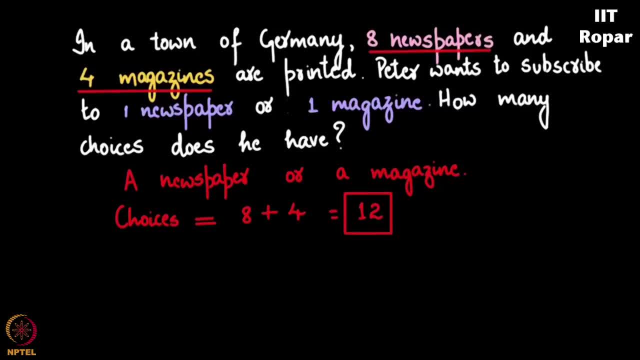 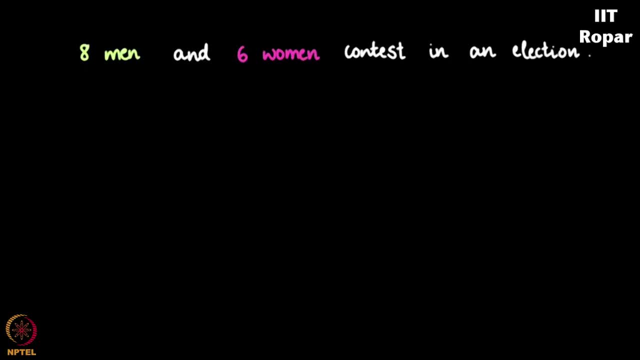 Let us move on to another example, where in a society, there are 8 men and 6 women contesting in an election. How many ways can the people choose a leader out of these? So there are 8 men and 6 women. How many ways can the people choose a leader out of these? 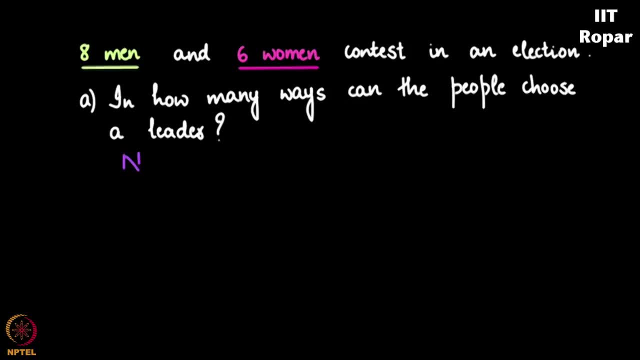 So there are 8 men and 6 women women- so the people have 8 plus 6, that is, 14 ways to choose from, because they wanted just one leader and hence it is a plus operation here. what if the people wanted two leaders? 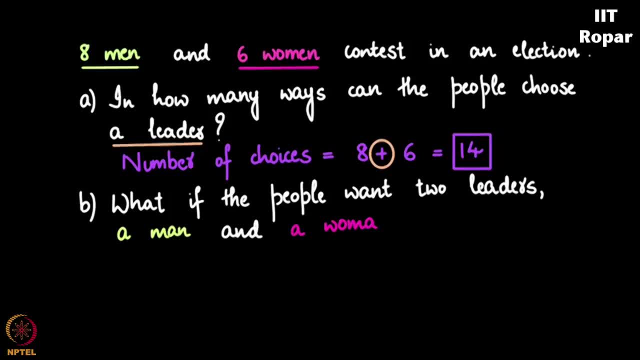 a man and a woman. I hope it would be very obvious to see that it would be 8 into 6, which is 48 choices. if they want precisely one leader, then it is 14 choices, and if they want two leaders, a man and a woman, then it is 48 choices. 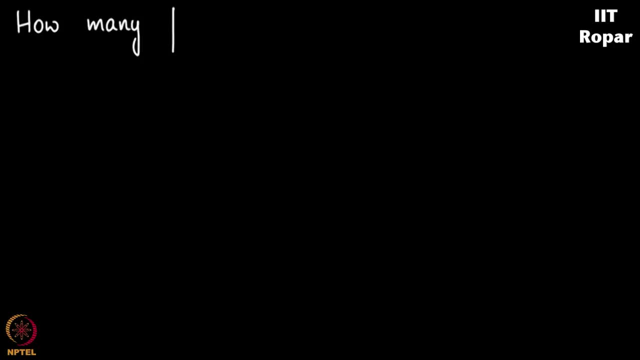 Let us move on to another question: how many positive divisors does 2000 have? before going to the answer, let me make it very clear what is a divisor. A divisor is an integer which divides another number. with examples it will be more clear. consider: 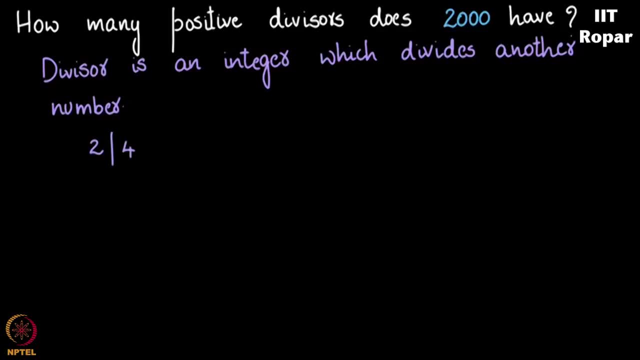 the number 4,. 2 divides 4,, 1 divides 4,, 3 does not divide 4, and 4 also divides 4, so you see, these numbers 1,, 2, and 4 are the divisors of 4,. 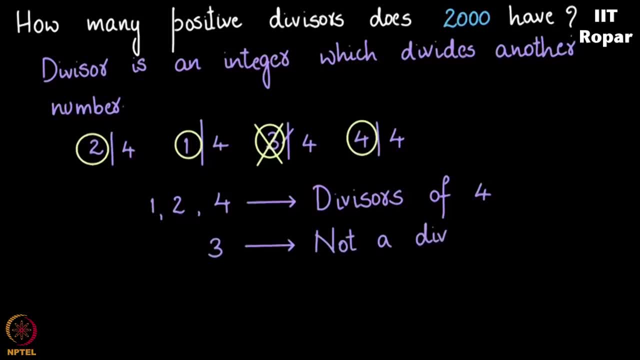 and 3 is not a divisor. What's the divisor of 4?? Because it does not divide 4,. 5 divides 10, hence it's a divisor of 10, divisors are also called as factors, so let us get back to the question: how many positive divisors does? 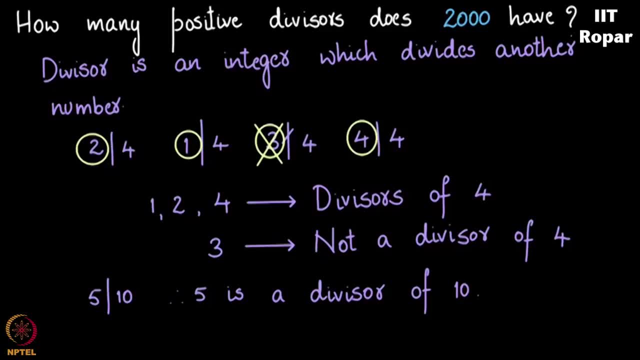 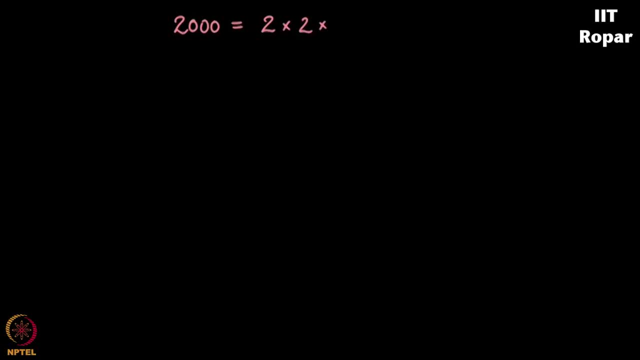 2000 have. Let me write 2000 as a product of its prime factors. so 2000 is equal to 2 into 2 divided by 2.. into 2 into 2, into 5, into 5, into 5, yes, so this is equal to 2 to the 4 into 5 cube. so 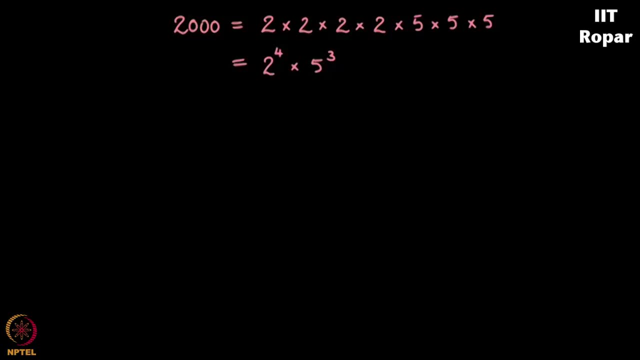 this is same as 2000,. so we see that divisor of 2000 must be of the form 2 to the A, into 5 to the B. now you see these A and B. they must be integers where A lies between 0 to. 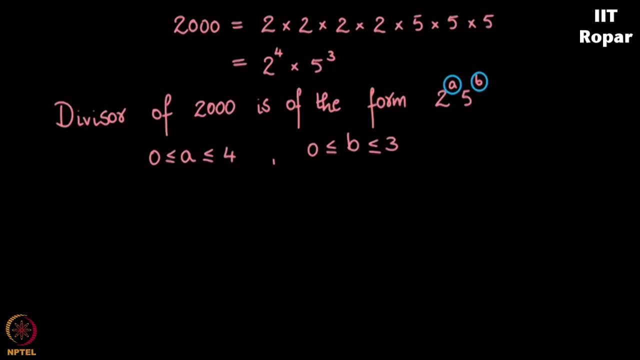 4 and B lies between 0 to 3, so A and B lie in a particular range. now, how many divisors do we get? We can answer this question by checking the possibilities for A and B. How many divisors do we get? 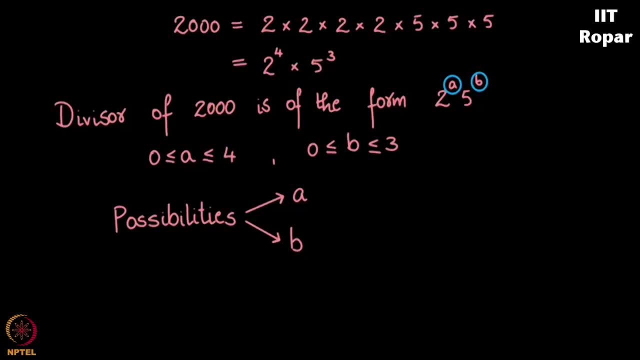 We can answer this question by checking the possibilities for A and B. So you see that A has 5 possibilities- 0,, 1,, 2,, 3, and 4, and B has 4 possibilities, that is, 0,, 1,, 2, and 3, supposing A takes the value 0, so 2 to the 0 will be 1, then B can take. 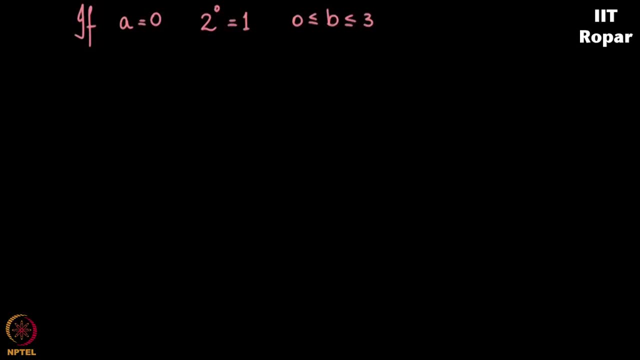 any value from 0 to 3,, 5,, 25,, 125, and also 1.. So all these are factors or divisors of 2000,. and if B is 0,, then this becomes 1, and A. 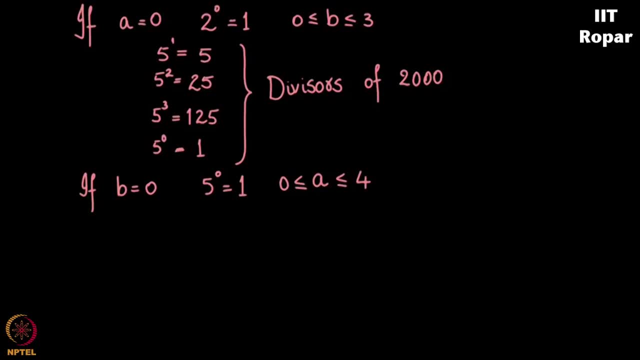 can take the values between 0 to 4,. let me just write some divisors of 2000,. 1,, 2,, 10,, 25,, 125,, 27,, 29.. Okay, and so on. so we have 5 possibilities for A and 4 possibilities for B. so how many possibilities? 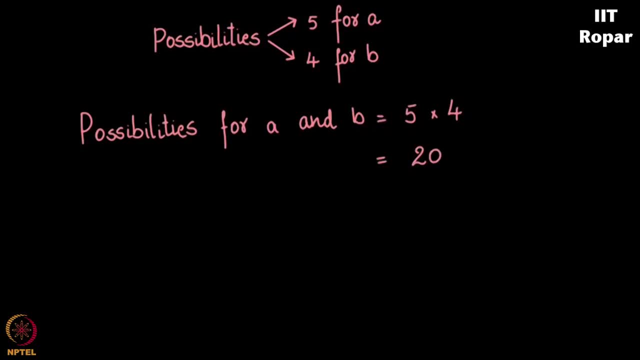 are there for A and B, It is precisely 5 x 4, which is 20, and this answers the question that there are 20 positive divisors for 2000,. let us now see another example. Charlie visits an ice cream parlor. 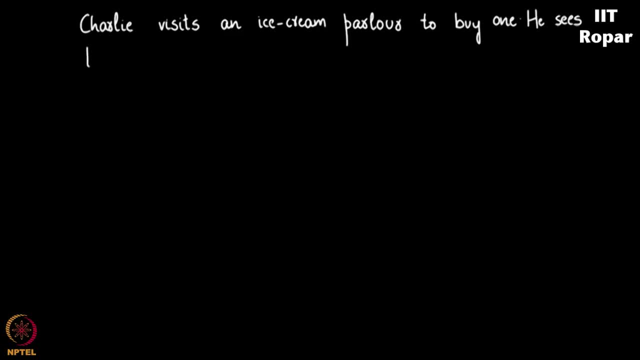 to buy one, and he sees that there are 3 types of cones, 4 flavors of ice creams and 2 toppings. so how many choices does Charlie have to buy an ice cream? Let me enumerate all of them, so let this represent Charlie. so he wants to buy an ice. 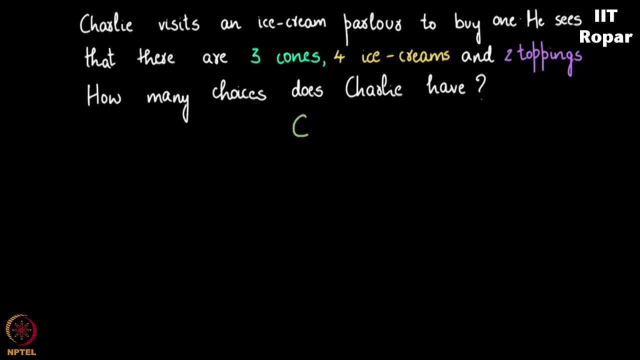 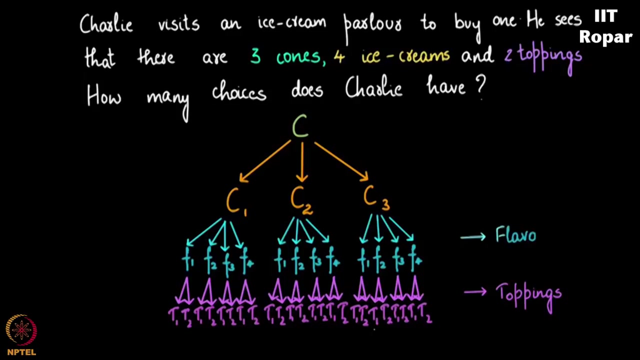 cream. he has 3 choices of cones and I will write them as C1,, C2, and C3, so for each cone he has 4 choices for the ice cream flavors like this, and for each flavor there can be 2 toppings. so this represents toppings and this represents flavors. so for this cone, 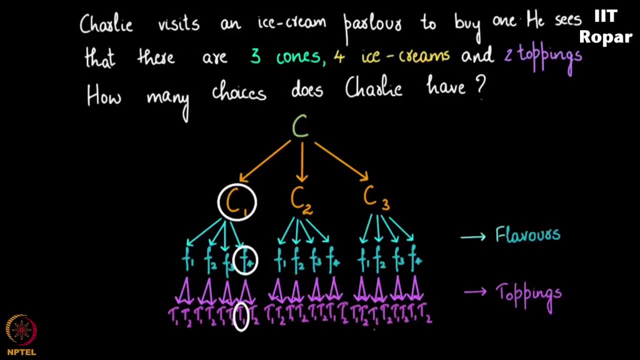 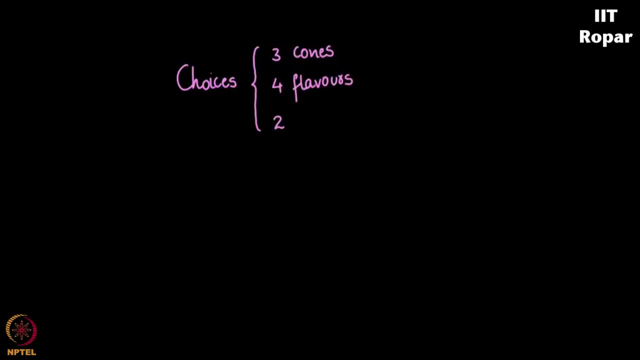 he can choose. What is this, This scoop and this topping, and so on. it continues for the others as well. so how many choices does Charlie have? He can choose between 3 cones, 4 flavors and 2 toppings. so you see, he must choose.